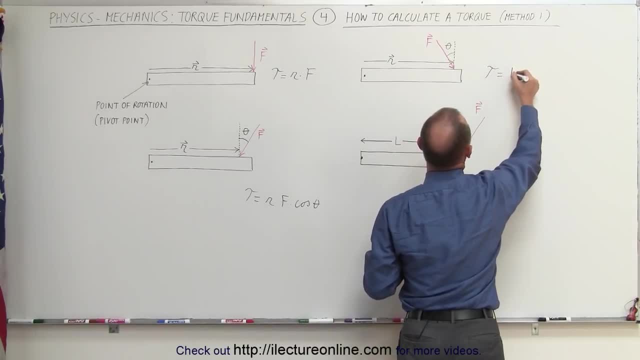 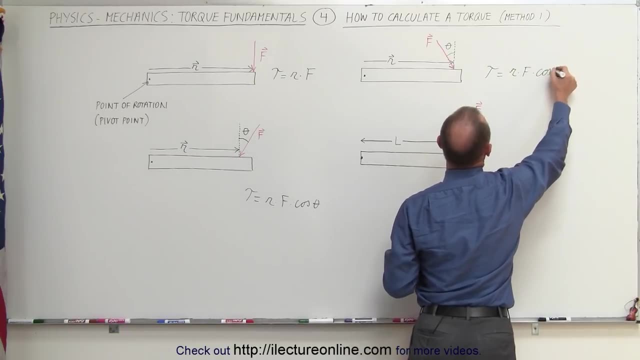 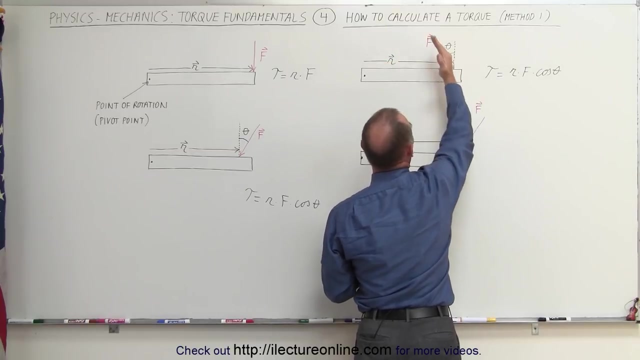 case you can say that the torque is equal to the force, or I should start with the magnitude of the position vector times the force, times the cosine of the angle between them. Again, we use the cosine because it's the angle between the perpendicular to the position vector. 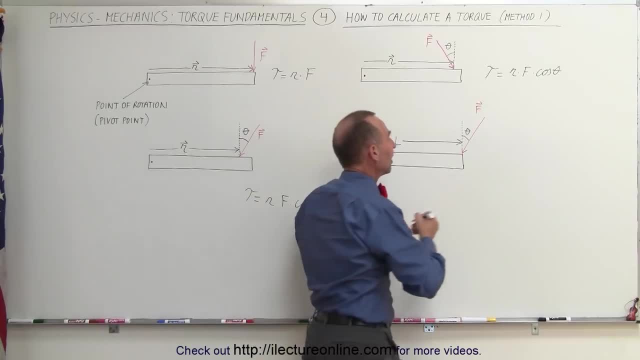 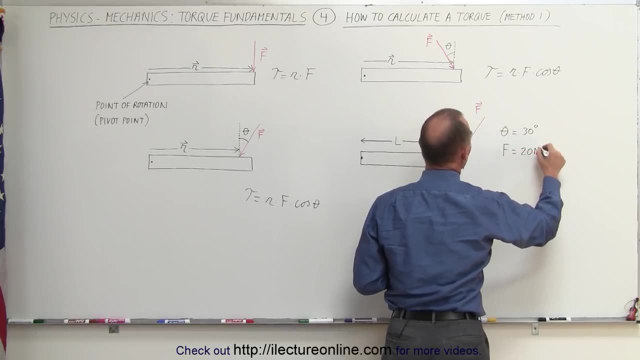 and the force. Now let's do an example. Let's say that in this case the angle theta is equal to 30 degrees. Let's say the magnitude of the force is equal to 20 newtons, And let's say that the length of this piece, here, the length of the object, is equal to well. let's 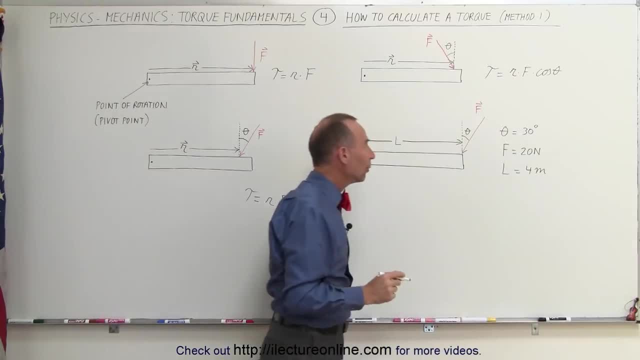 call it four meters. How do we find the torque caused by that force? The torque would be equal to the length times the magnitude of the force times the cosine of the angle between vertical, the perpendicular to the position vector and the direction of the force. And so 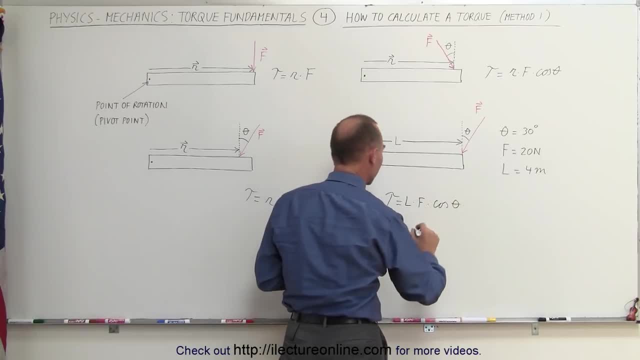 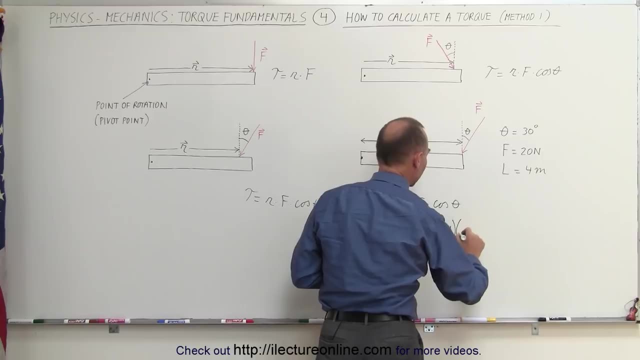 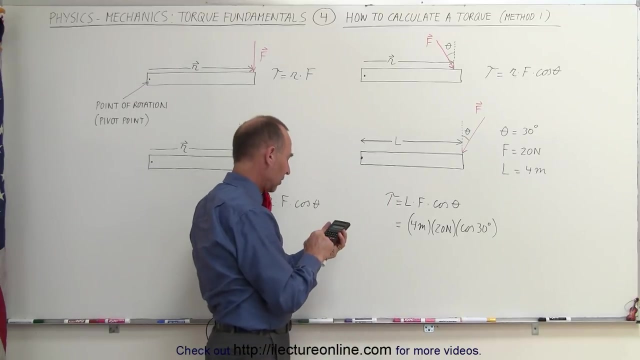 that would be the cosine of the angle theta. In this case we take the length, that would be four meters, we multiply it times the force, which is 20 newtons, and then we multiply it times the cosine of 30 degrees, which is about 0.866.. So we get four times 20 times the cosine. 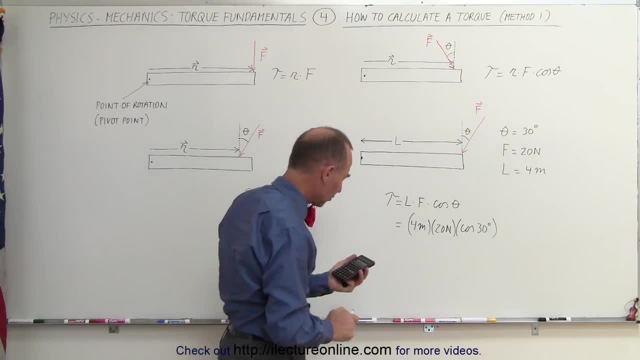 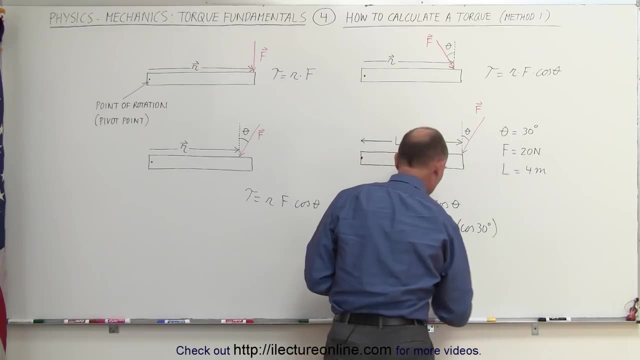 of 30. And we get 69.3.. We'll just round it off: This is equal to 69 newton meters. Notice that the units of torque is newtons times meters, which is force times distance, And so in this case, the torque. 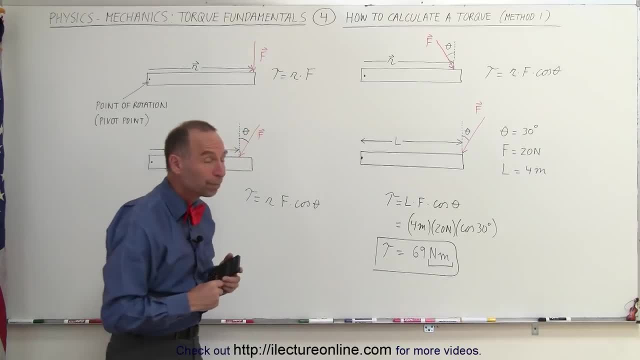 would be equal to 69 newton meters, And that's how it is. That's our first method of how to find the torque here. Notice, we're only dealing with the magnitudes, not with the actual direction. So we talk about it in terms of magnitudes. 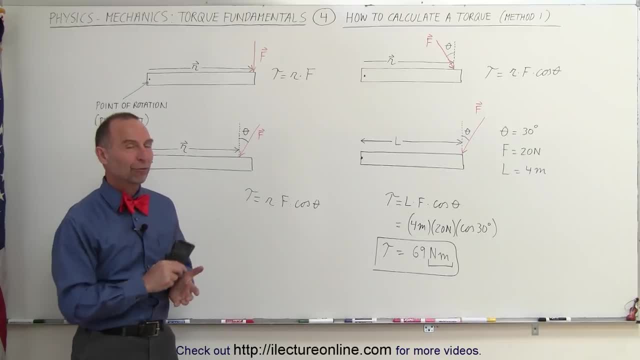 And that's in terms of vectors that will come later. That's our first method. On to the next one,